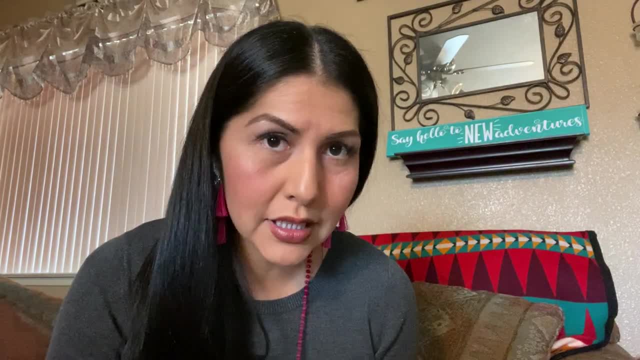 I then go into another section called Making Local Connections, and this is the part that I'm finding that is really important. I'm finding that there's a lot of people who are making local connections, so that's something I'm finding with the music educators When you're coming and 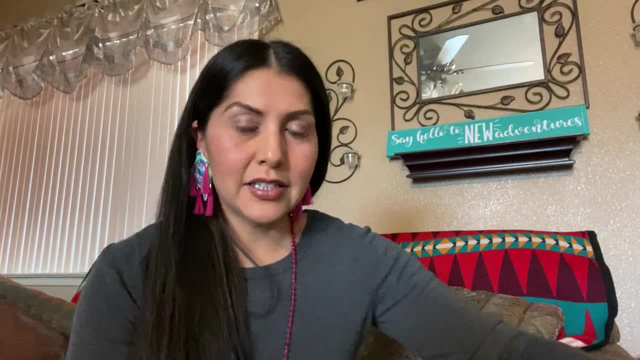 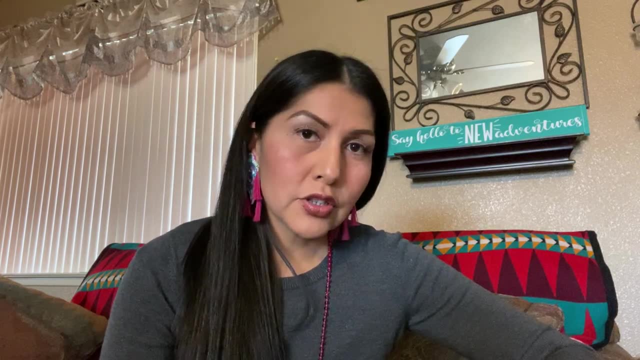 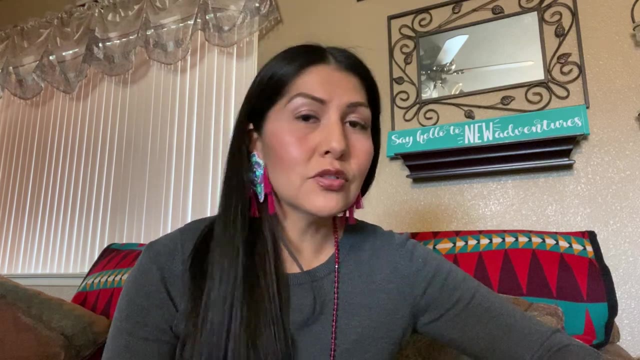 commenting on forums. it's almost as if this is the last step that you want to do, which is actually talk to the local tribes. So when you talk to the local tribes, it might be best to attend events first, and it's really important to establish relationships When you just go into a Native 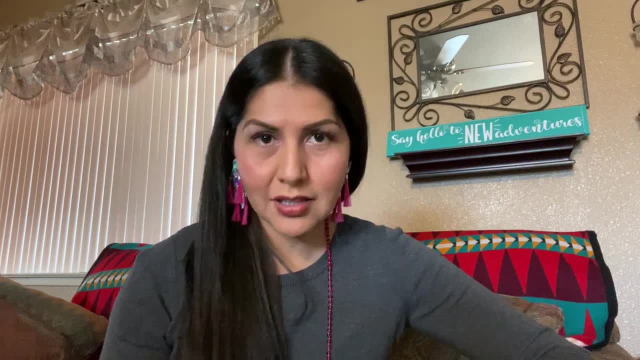 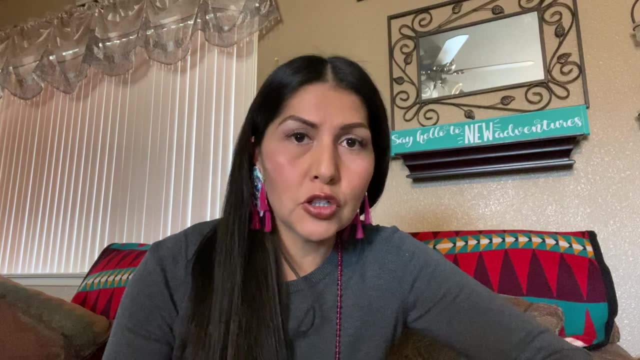 community, or you're like: I just want these songs because I want to be able to say I'm a culturally relevant educator. I heard you need to start with the First Nations people, you need to do a, a land acknowledgement, then maybe go get a song. I'm going to go meet this and I'm going to go get. 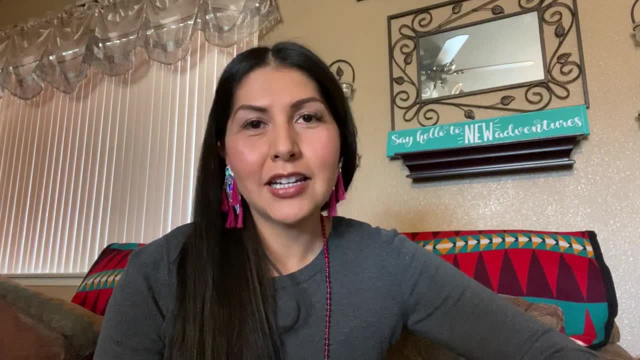 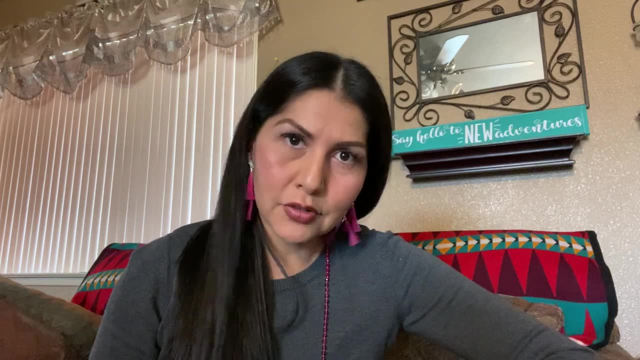 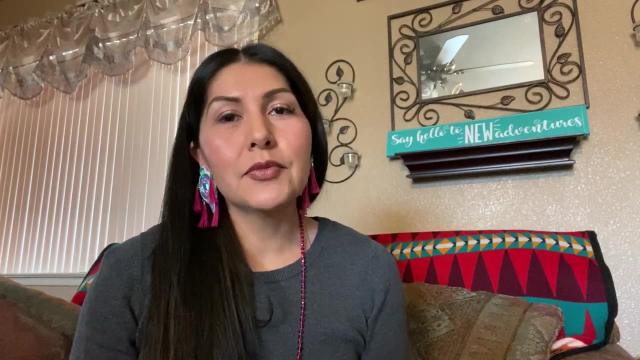 this. The problem with that is that that's exactly how Native American people have been treated by colonialism throughout the entirety of this country. Let me go get things from you so that I can benefit from them Now as music educators. there's a whole other aspect to this that I did. 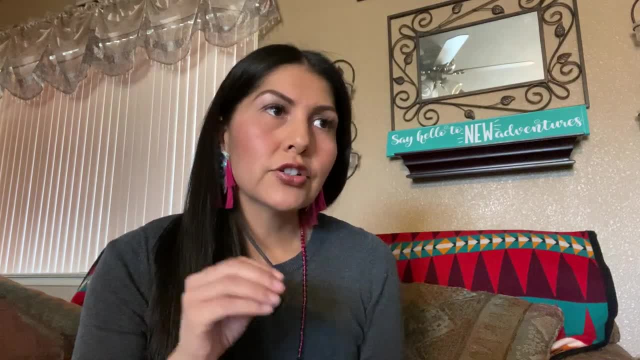 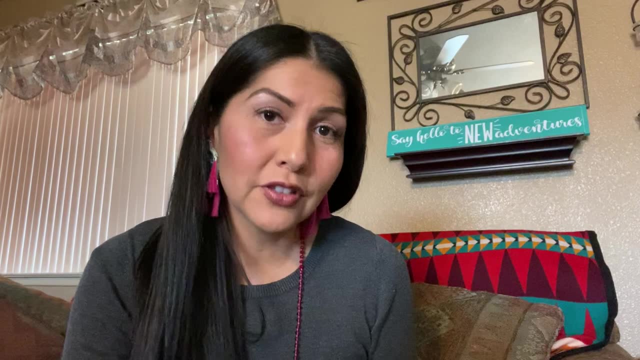 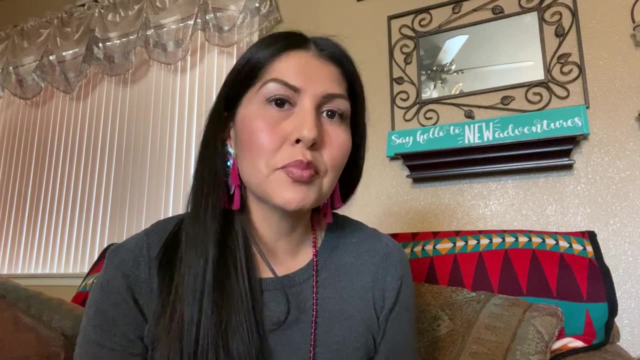 not touch on in my article in this book, and that is understanding cultural music versus classic music. right, They have different functions. Classical music has a different function than cultural music does. Classical music isn't the identity that most people kind of look for When 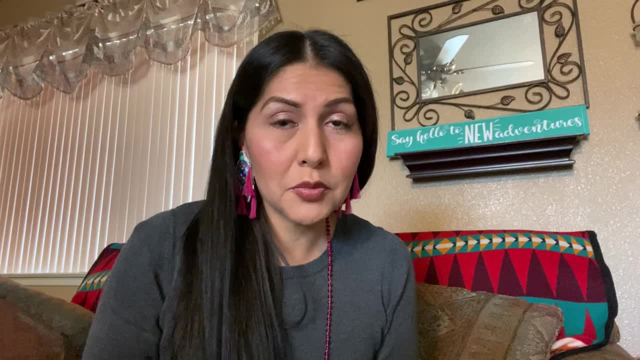 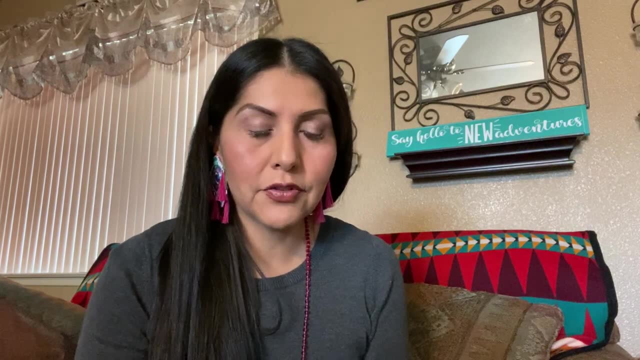 you meet new people from other nations for myself so, I'm Pyramid Lake Paiute. if I'm going to share a song from you, from my culture, from my identity, it's going to be a circle dance song from my tribal nation here. 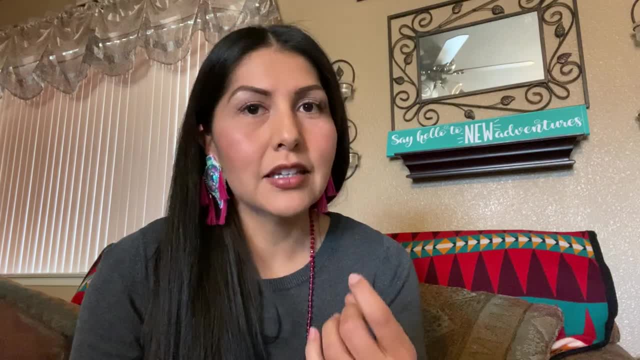 Either in the languages of Washoe, Shoshone or Paiute. And then you know, if you say that, oh well, I don't have a culture, or I'm a classical musician, well, are you going to share with me? 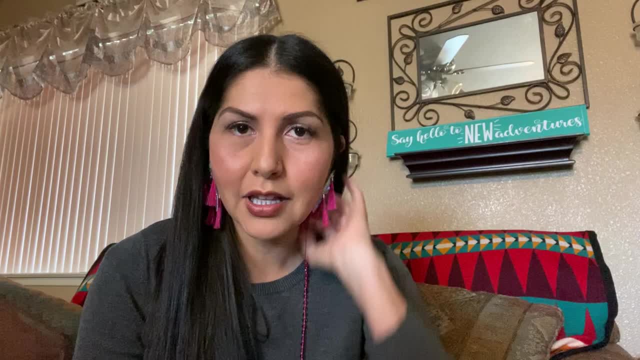 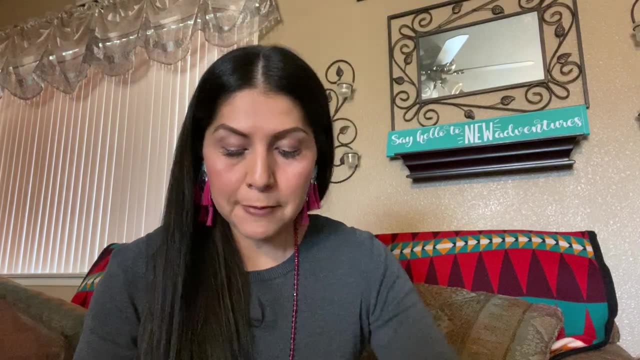 then Is that going to be your idea? Are you going to be able to exchange a song with me from the classical music genre and say that that's your identity? No, because they're two different functionalities, right, And so I don't get into that in here. So making local connections is a 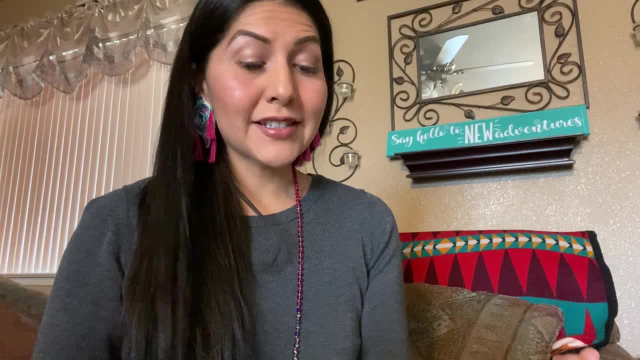 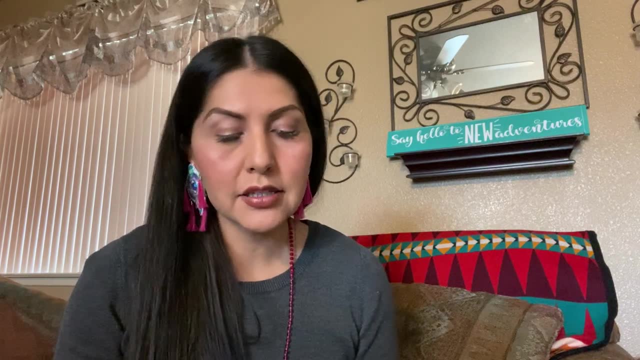 whole section. I have one, two, three, four categories on that. Sources for authentic music and dance. This is another hot topic, I believe, anytime we're talking about any culture- And you notice I'm talking about cultures, right, When we say Native. 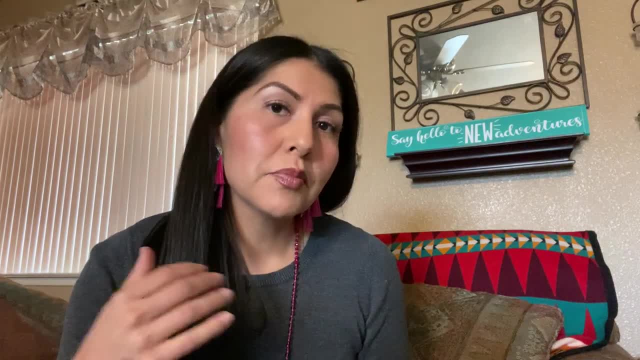 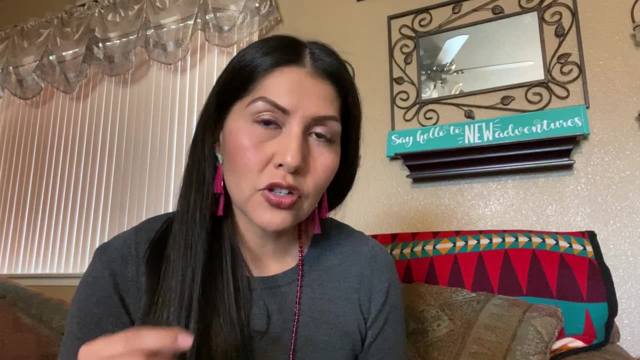 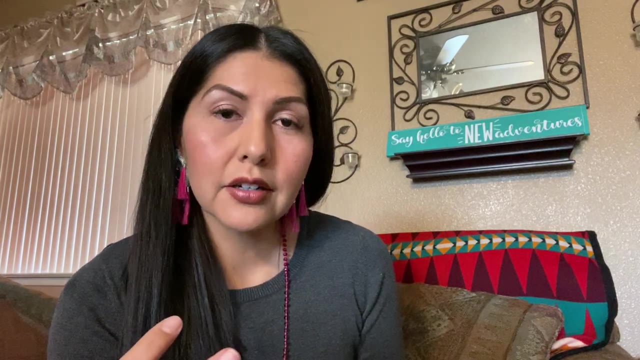 American. there's 573 tribes. within that. There's also a powwow. there's the powwow trail within that powwow, music, dancers and everything. Then there's your specific tribe by tribe dances, songs and things like that, And I always also hear. well, some of the music isn't. 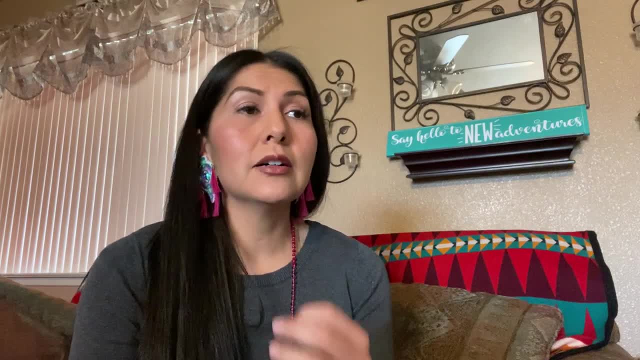 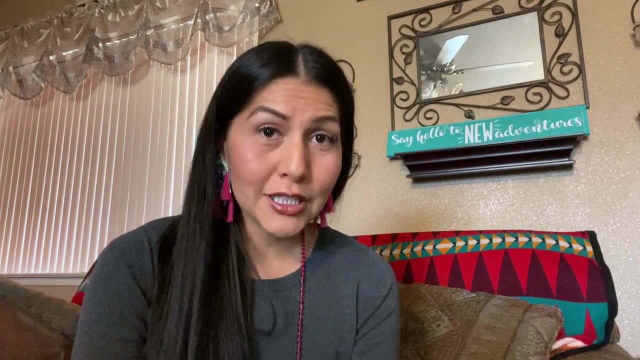 allowed. It's not allowed to be taught in schools. It's just so sacred. Well, that's only if you go. you know, if you're looking for things like that, there are musics in every nation that are not sacred. And how do I know this? I know this because I'm around. I go to Native conferences. 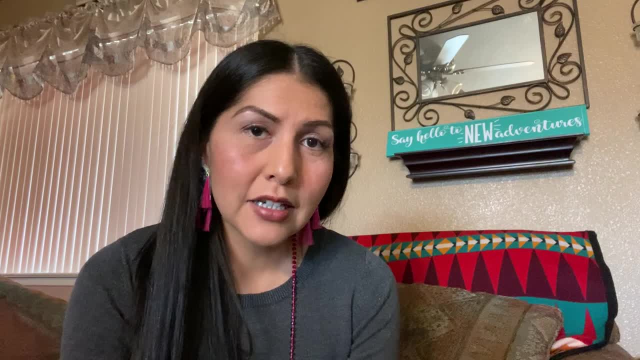 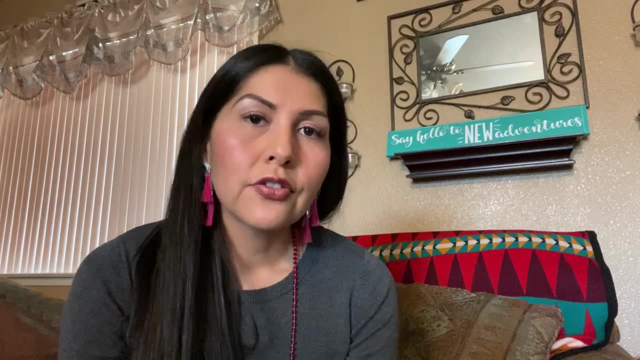 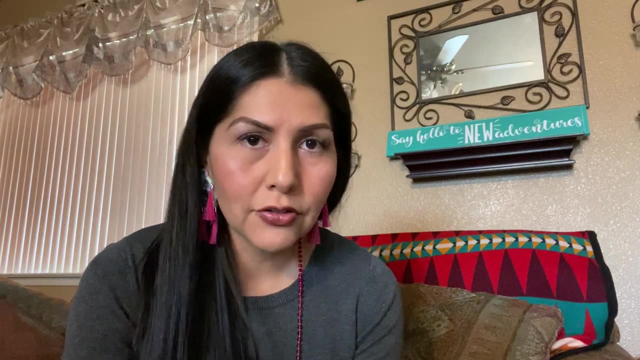 with over 200 nations represented there, and they have a cultural night And during cultural night, the youth or adults, or whoever it is, share songs from their tribes. So they're not going to share something that's super sacred, That's like only meant for members only When they share, when we share from tribe to tribe. 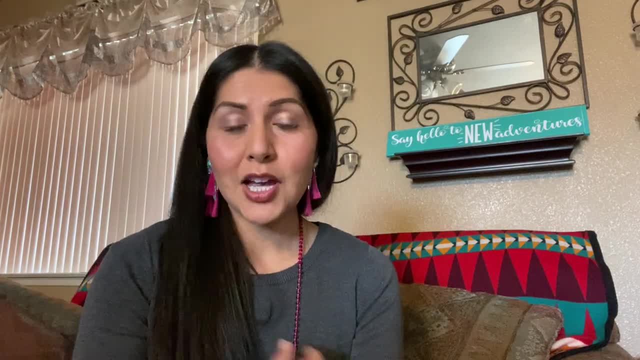 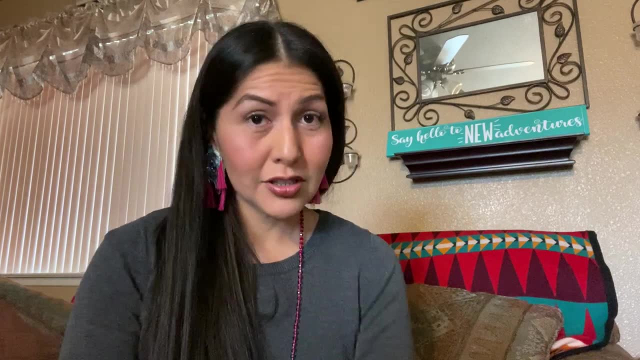 we know what songs we can share from tribe to tribe, But I spend time in these environments all the time. I meet culture bearers from different tribes. everywhere I go, I start the conversation and I'm used to starting the conversation. I don't go into these communities. 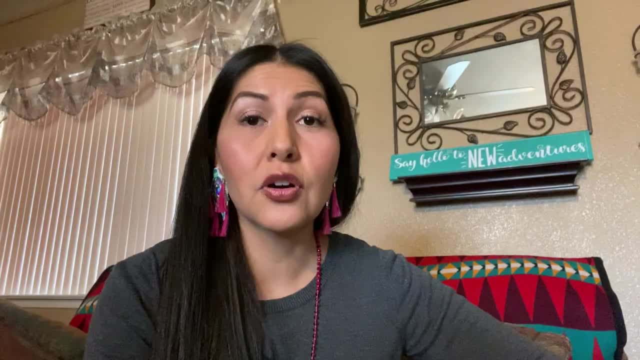 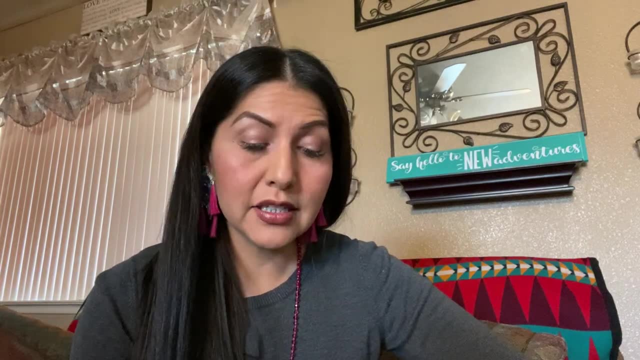 or any other cultural community for that matter, and want to know: can you tell me your history and demand that That's another part to music educators? I think that we need to definitely build in is: how do we share- And I think that's another part to music educators. I think that we 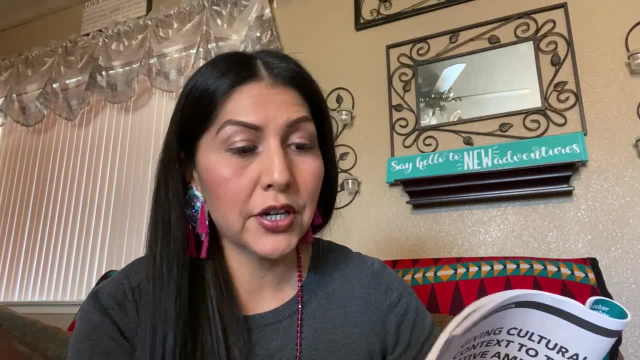 need to definitely build in is: how do we share- And I think that's another part to music educators. I think that's another part to music educators. I think that's another part to music educators- how do you find these? So one? I'm going to read you the first paragraph from the sources for 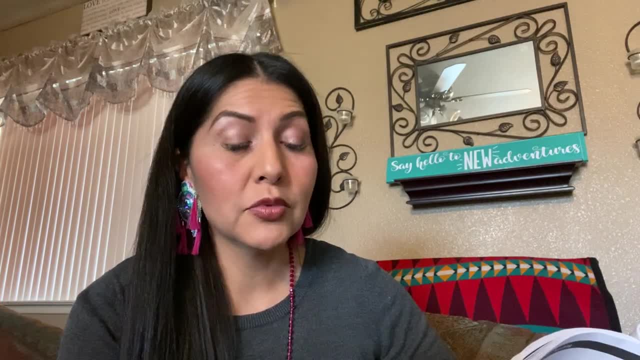 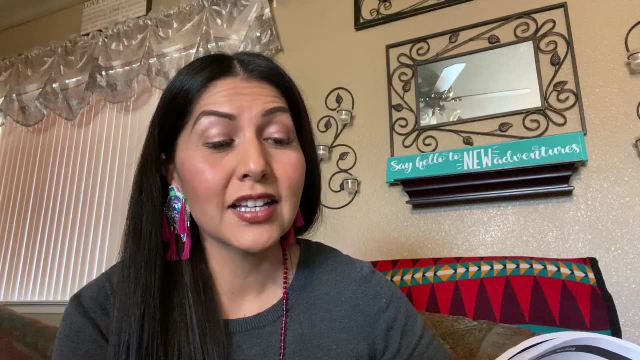 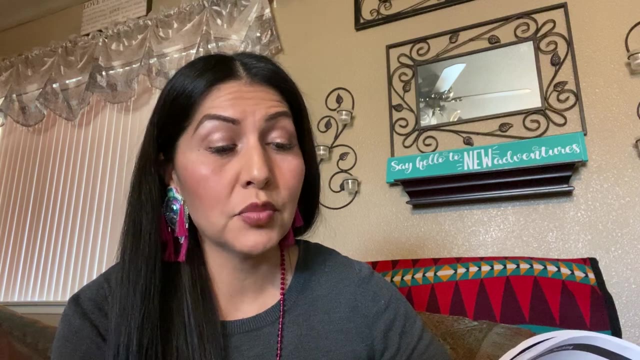 authentic music and dance Says. most of the songs used by tribal nations are fun, simple tunes that are used for social dances, annual events, honorings, seasonal celebrations, lullabies and ceremonies. ceremonial music that is sacred will not be given out by an actual culture bear. 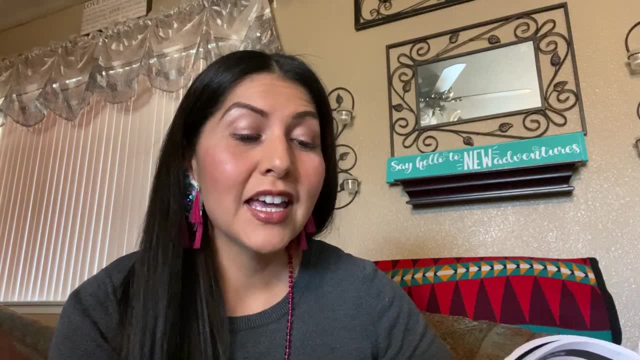 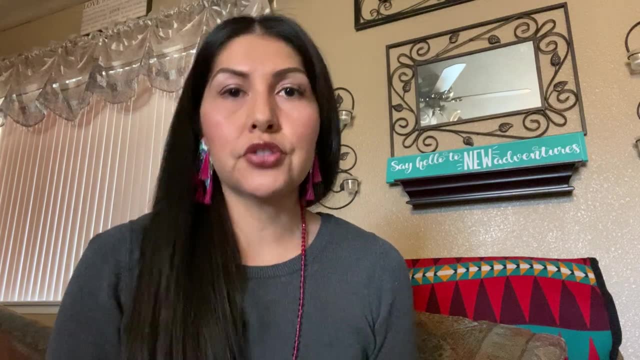 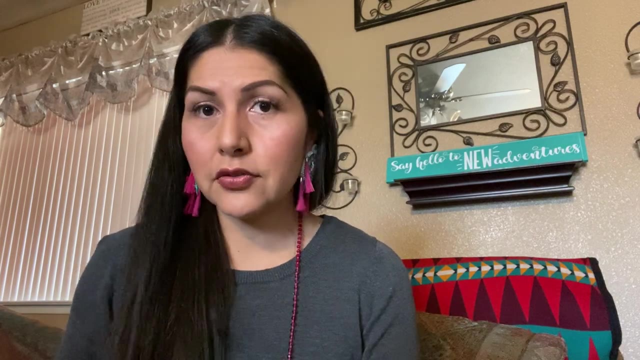 of a tribal nation because they know the cultural protocol and understand what should remain sacred Um. the protocols are extremely important to follow, And so that means this is not taught in music education on how to approach different cultures, not just the Native American cultures. 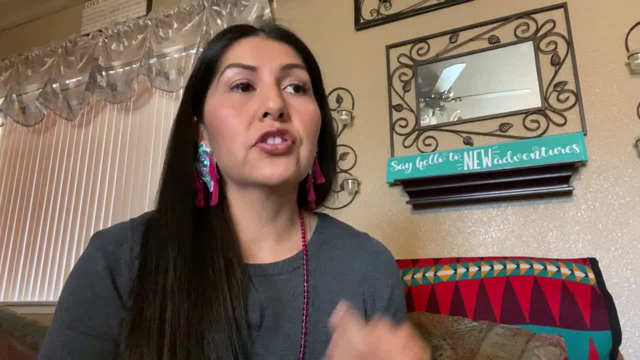 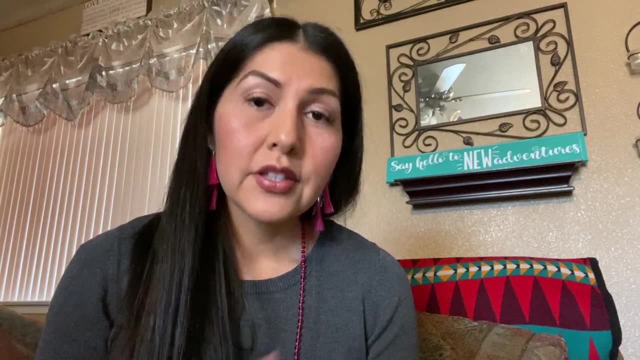 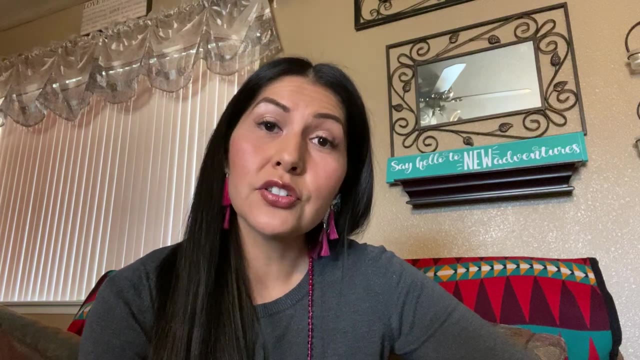 but how do we, how do we then form relationships with the culture we're trying to learn music from? And I do also have to stress that this takes time. This takes time. You need to spend a certain amount of time with people from their different cultures, Otherwise, you could just say that you're 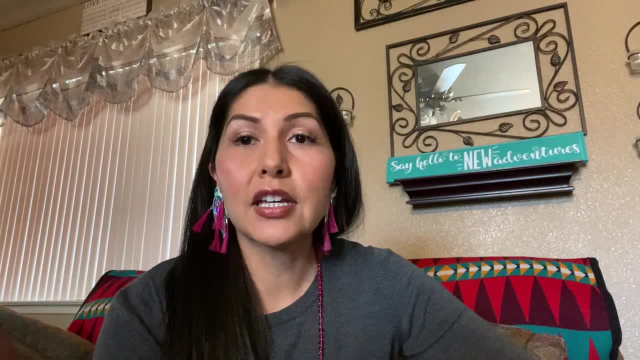 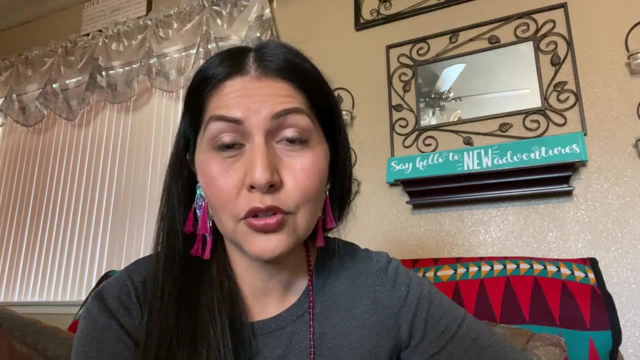 going to spend most of your time with classical music. Um, I hear a lot of educators say: I don't have time to travel, I don't have time to do this, I don't have time. In the United States, we have a lot of people from around the world who are living in the big cities, or any cities. 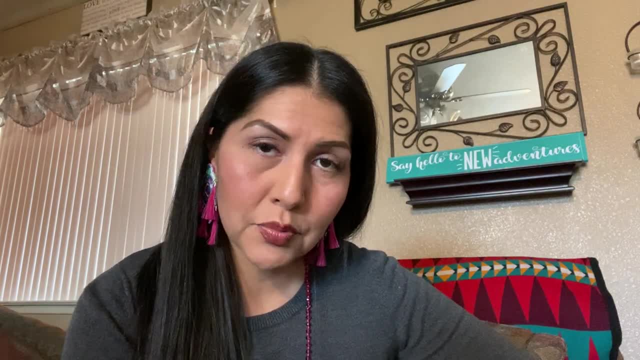 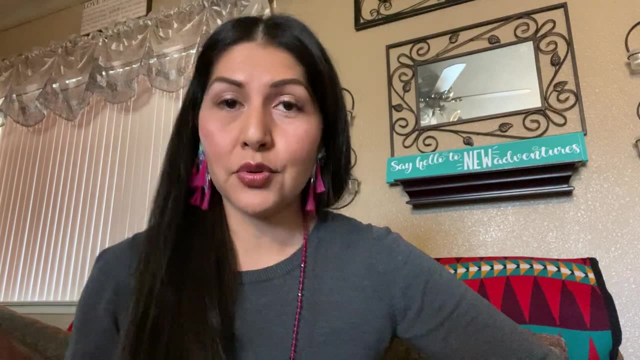 closer to us. If we spend time getting to know those people around us- um and again, it takes time- That'll deeply heighten our ability to understand Protocol uh from other cultural groups, especially Native Americans, rather than. 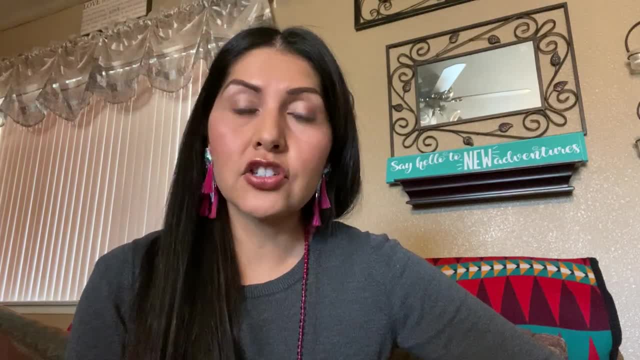 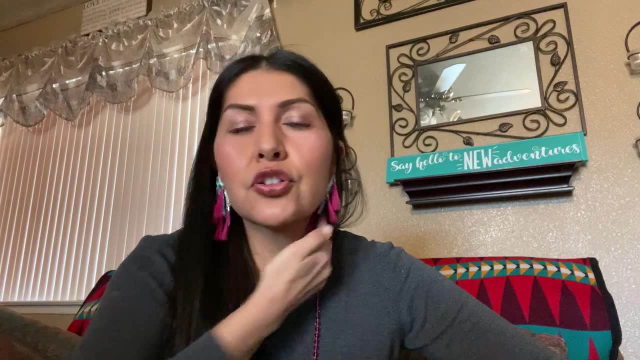 can I have a song? I'm trying to be a culturally relevant educator. Can I just have a song? I was told that if I do this and again this, this whole idea that there's one, there's certain phrases that you need to say to get what you want, That's very. 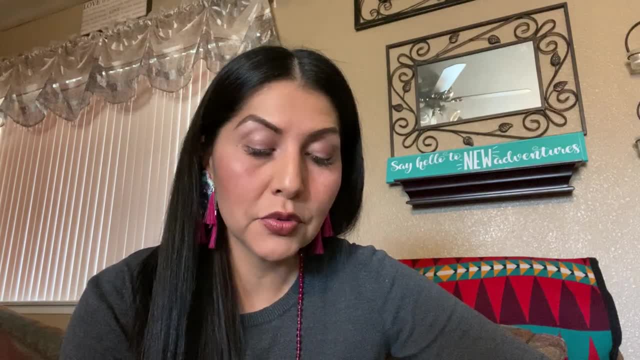 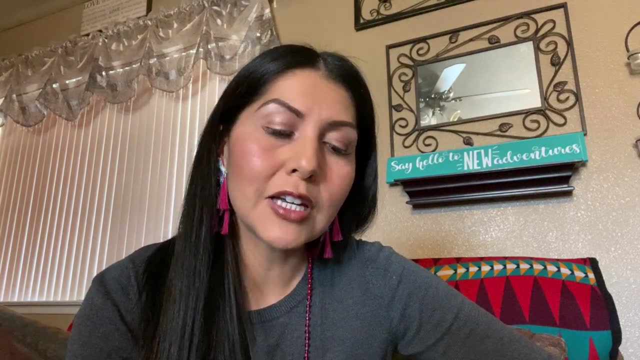 it's very much a colonial construct. When you talk about cultural people, especially Native American music, um, our music is it's it's our identity, It's important to us. We do believe that people who are coming to this country, uh many tribal cultural bears, 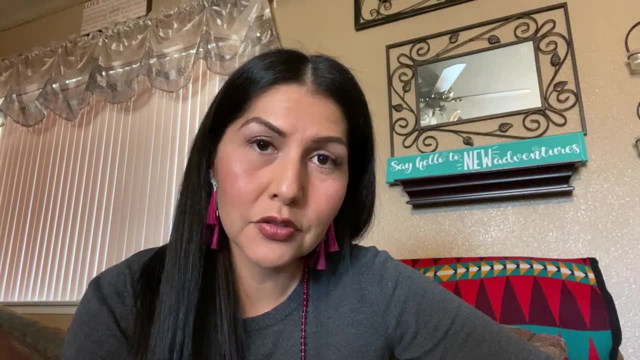 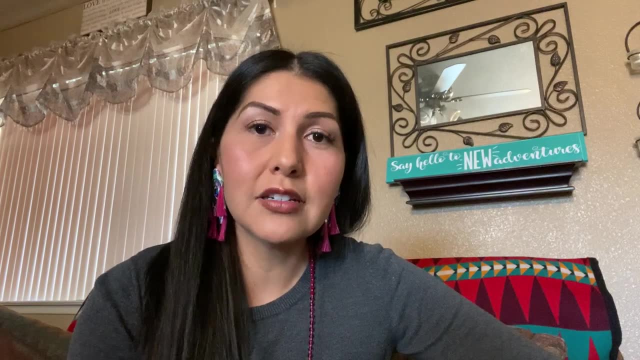 that I know they do believe that people need to understand and know our songs from the certain areas because we have ties to the land, no matter where they are over the United States. Um, and some people I know, there's about 13 different states in the United States. 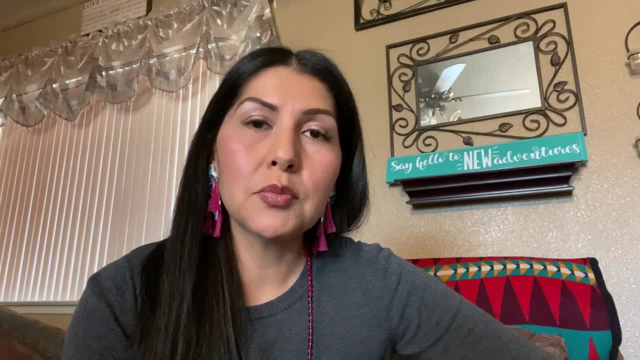 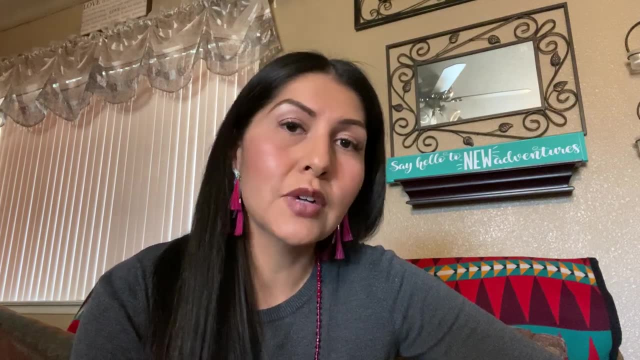 that do not have tribal nations. sometimes, Um, and some people will say that we don't have any tribes in our state. Well, do you know why that is? Most of the time, it's tied to capitalism. It's tied to who wanted to benefit from the land. So they push the people. out of the state. So there are people, uh, there are native tribes, who are originally from your state. They're just not there because if they were to be acknowledged, the government would have to give them back that land that they owe them, which is kind of the story of a lot of the different. 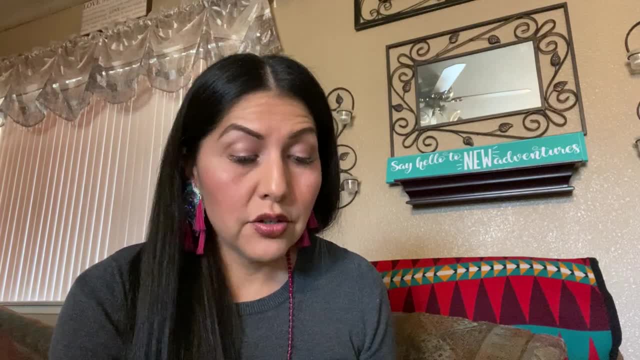 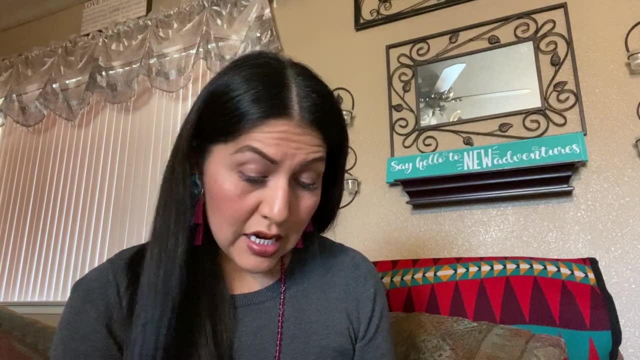 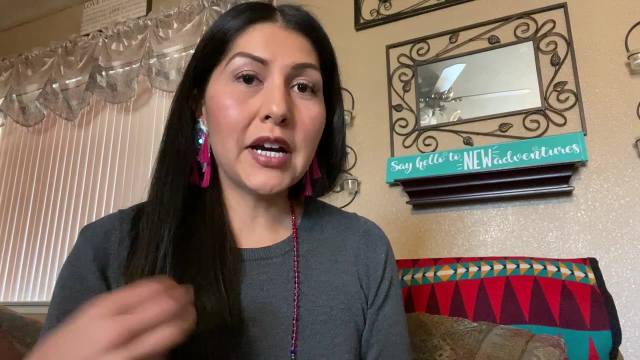 reservations um going forward. So again, sources for authentic music and dance. I have three, three different pound paragraphs there. uh, teaching Native American music with authenticity. Again, you cannot teach anything um, right now, my newest form of music that I am teaching is mariachi: right, Mariachi. 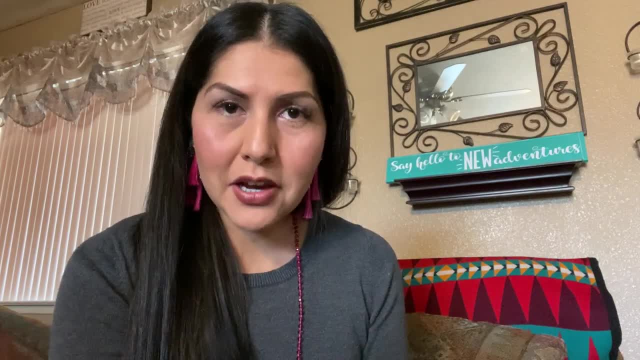 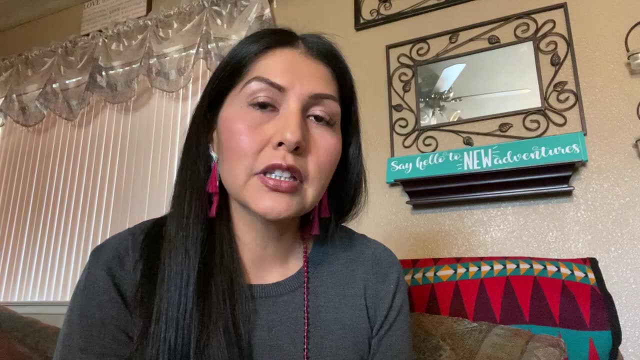 I cannot be a successful mariachi teacher unless I spend time learning about. what are the standards within mariachi music? How is it? How does the trumpet play? What is the relationship to the trumpet to the violin? What kind of tonalities are in this music? 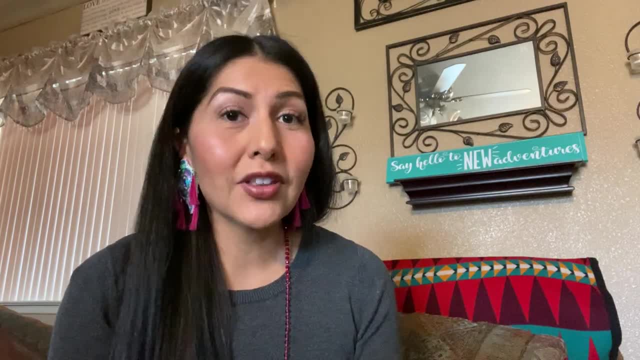 You know what is it used for, What events are used for. In order to do that, I need to spend time, hours and hours, hours at a time, probably these days. We're going to learn about some of those things in the future. 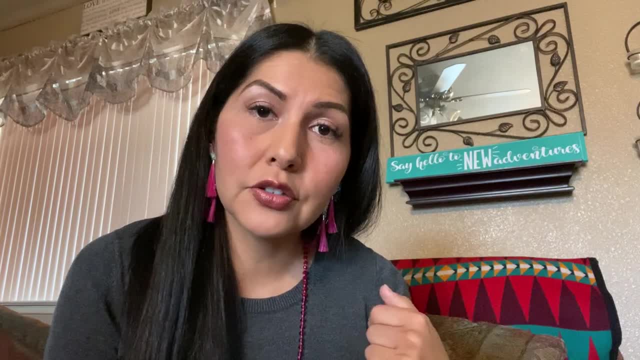 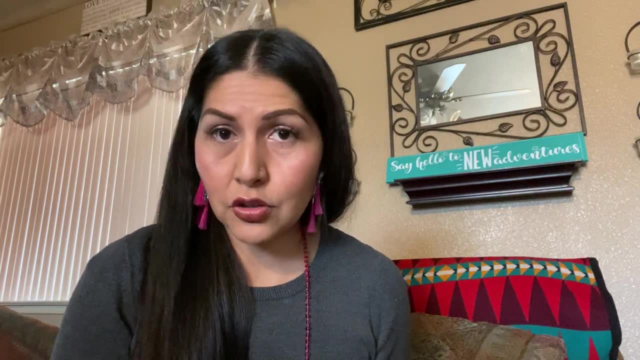 These days we're also busy, but hours at a time finding the experts in the area to learn from so that I will be able to successfully pass on the knowledge and successfully teach students in the right way in the culture- And I'm not culturally appropriating anything- 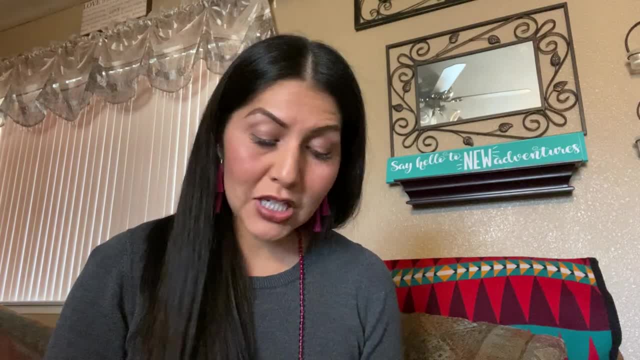 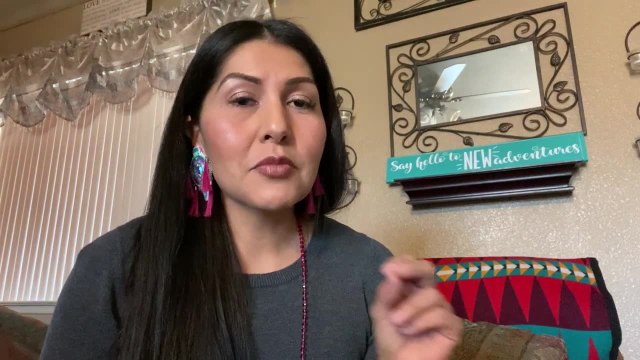 or giving misinformation. The same thing especially applies to Native American music. Um, when you're trying to teach anything with authenticity, the le the less amount of time that you spend with it. Michael, I just heard the song. I just want to listen. give me the music and 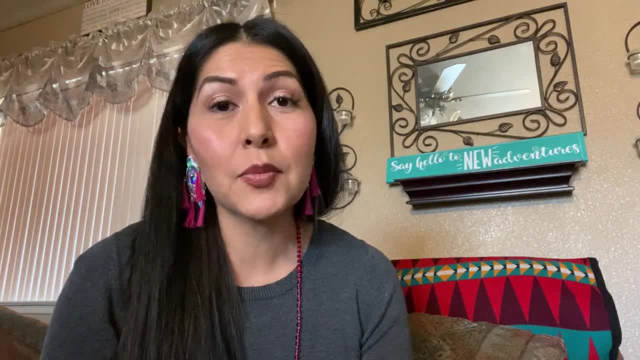 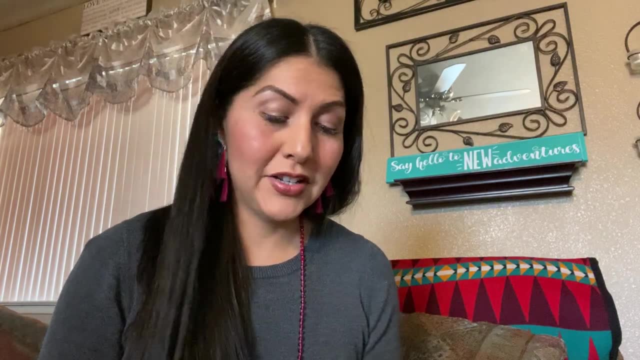 then i want to learn it. i don't want to learn anything about context, i don't want to see how it happens. um, that is not teaching any cultural music. uh, culturally and not authentic actually, it's actually kind of more kind of being appropriate, appropriated or just rushed over. 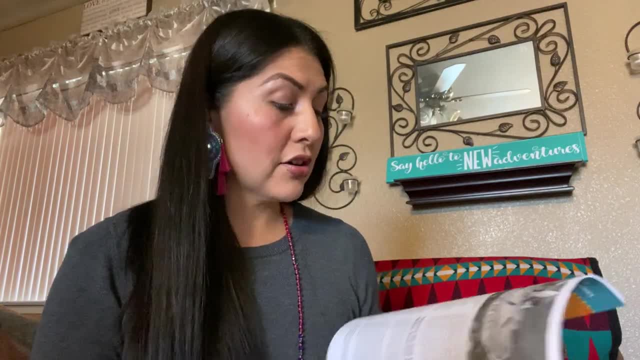 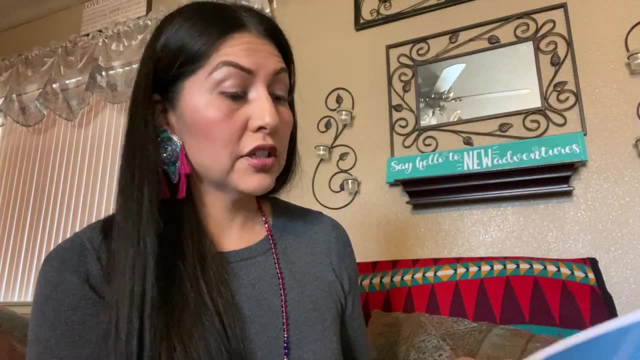 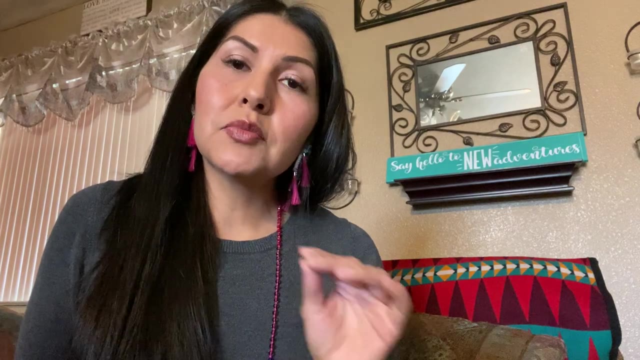 and the last part i have on in this article. so when the teaching native american music with authenticity? i have one, two, three, four, five paragraphs on that. and again, this article is an activate magazine and on the decolonizing the music website, if you go into some of the 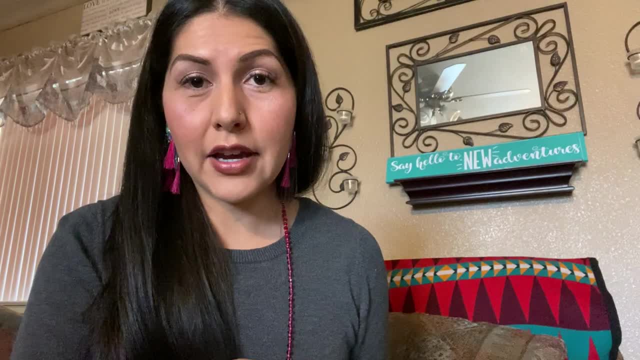 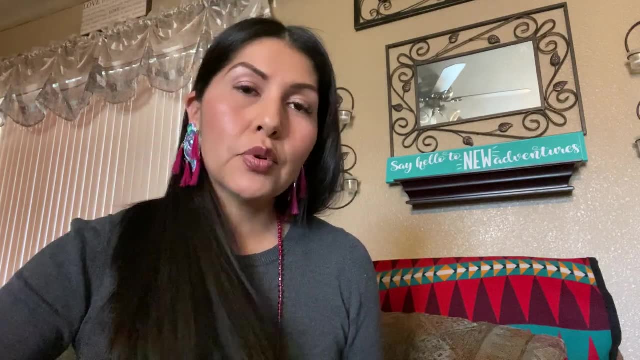 articles you may find. also, i did do another article on that website. it's not in the same order, so to speak, but you will still find the information there and this is really important to read through. so everything i'm writing from is from a first-hand experience. i'm not an outsider. 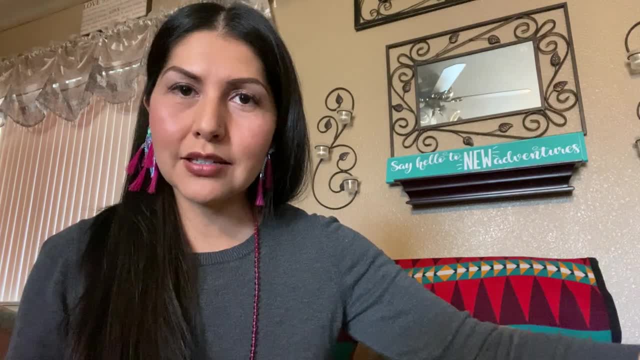 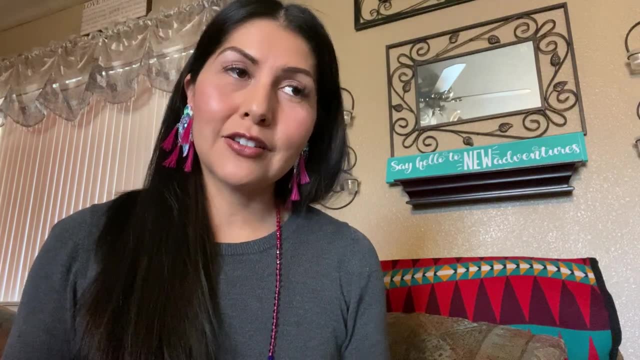 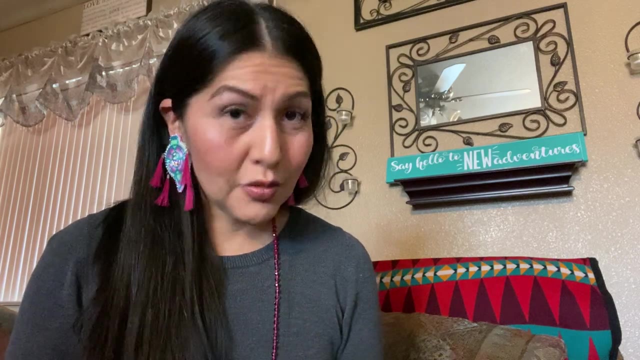 looking into the culture, writing about how i think the culture is. i am an insider knowing exactly what the culture is. trying to explain to people who are outsiders: how how to approach the music and, definitely for music educators, how to how you need to be able to do this and do this correctly. there is 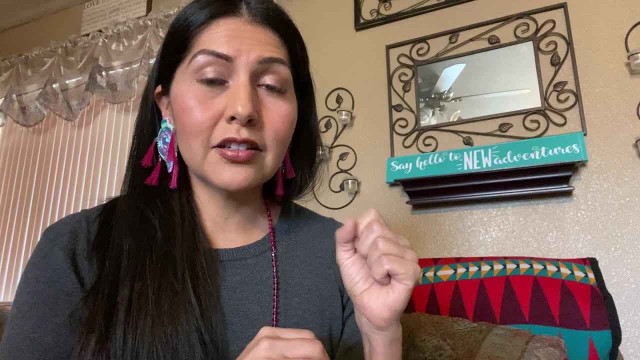 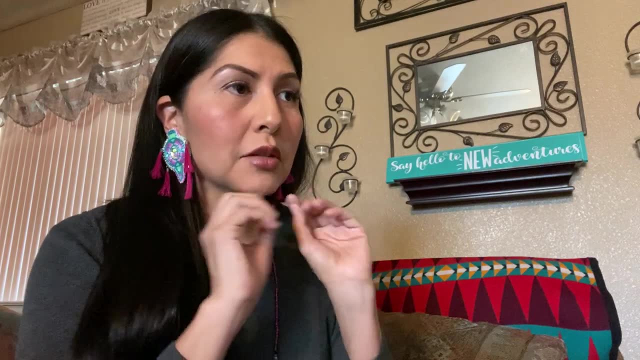 a culturally appropriated way. there is a i'm gonna, i'm gonna colonize this, which most of our music has been done. i want to write it down. um, i want to get native flutes out and i want to put music in front of me and i want to write it down, and i want to write it down, and i want to write it down. 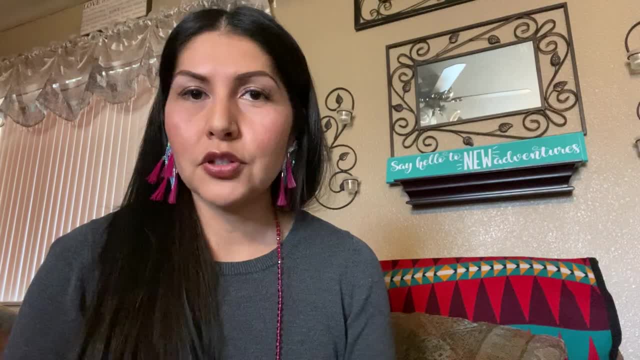 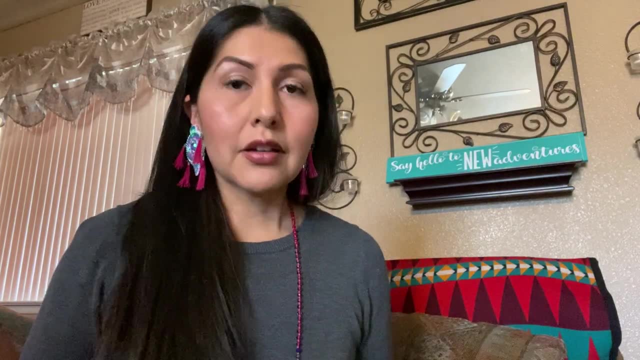 and a native flutes, and you know that those are not culturally appropriate. those are not culturally relevant, right? those are different pedagogies, those are colonized thinking and so when we decolonize something, usually you need to go to the source. then the source usually is a: 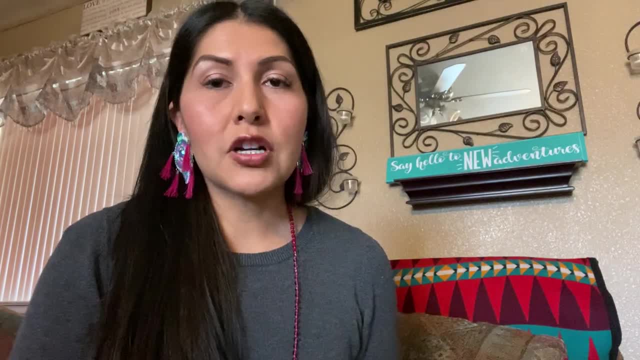 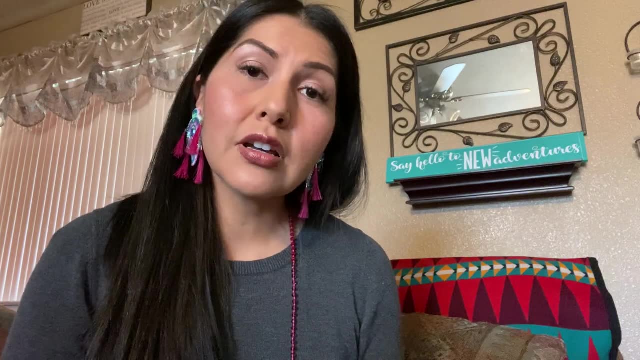 person, from whatever culture, from whatever tribe, from around the world, who is a culture bearer, who does practice the music, who has spent hours and hours and hours in different communities and knows um a vast majority of songs, who knows a huge variety and has a lot of experience with. 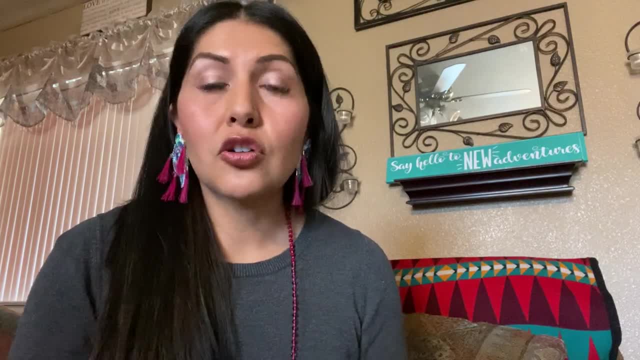 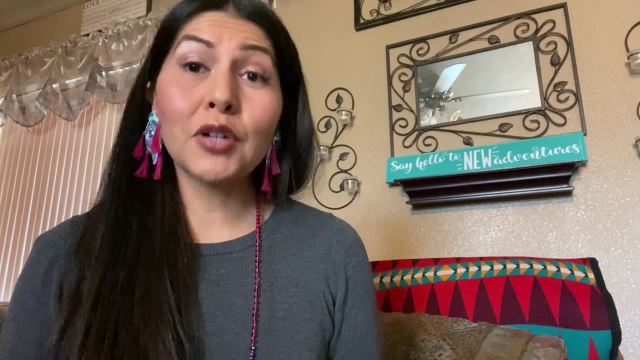 seeing so many different um ceremonies, knows what is sacred, knows what is not. so you need to find the experts, primary resources in music education, so many people have told me. well, i've been using primary resources. you mean printed books by people who are not indigenous. uh, academically, 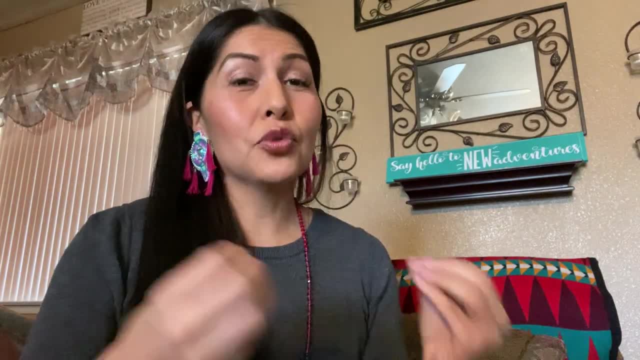 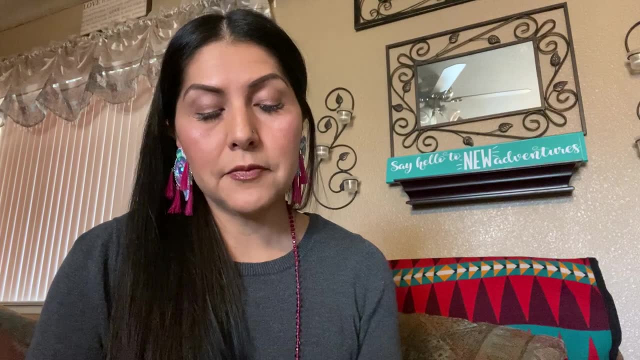 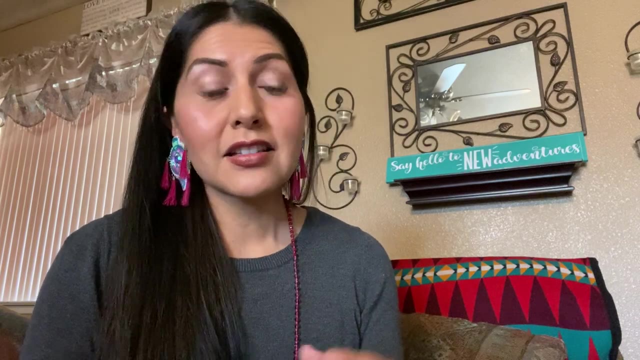 speaking correct, those could be primary sources, realistically speaking, unless it's coming directly from a tribal person or a native american or, um, anybody who practices their culture. if they're not a culture bearer, they don't do these things on a on a on a regular basis, right, those papers are. 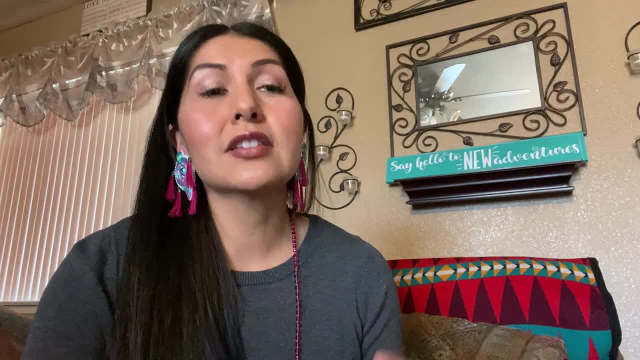 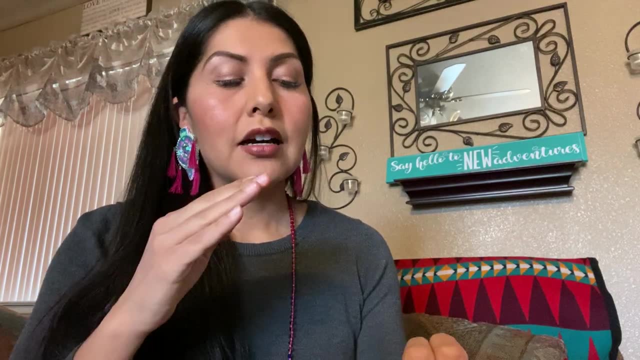 they're just papers. i'm not going to consider that a primary resource and i'm not going to allow you to to hold that up and say that yes, this is me, i'm being authentic. you need um, an indigenous person, you need a native person with you to make sure that you're following the protocols and also to 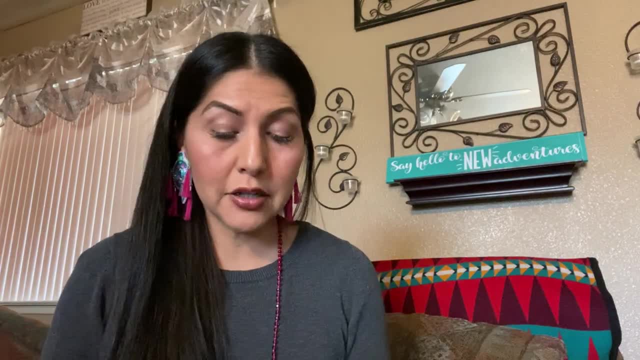 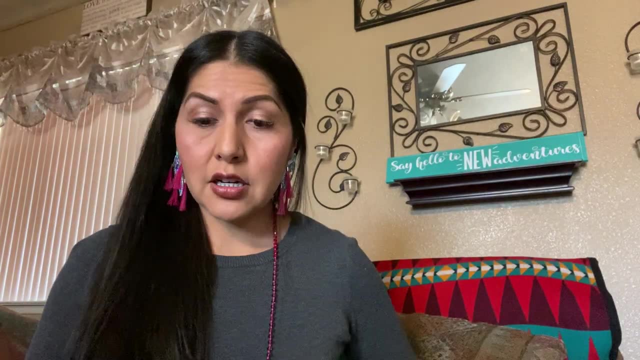 make sure that you're being respectful, not just a paper written from an outsider. and now, lastly, i will say um. and then it says: explore the vast majority of songs that are written by indigenous native american music. the closest um resource right now that is out there is louis bellard. 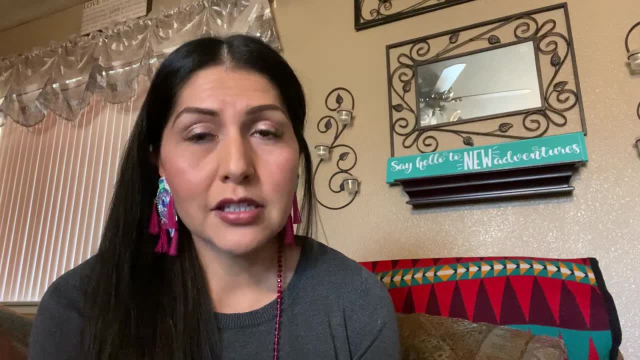 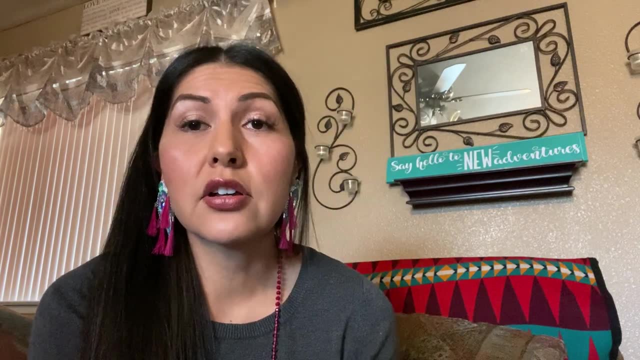 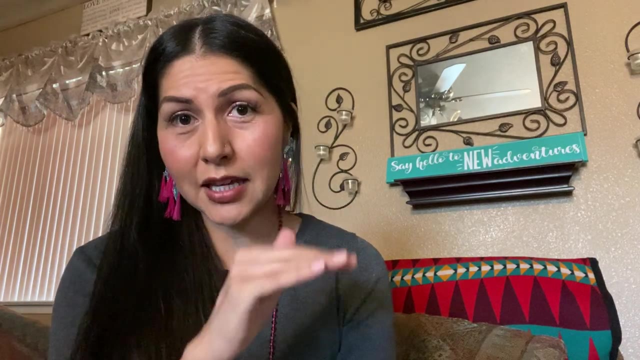 um, if you take a look at louis bellard, he? um was a native american composer and he collected songs. he does have a. there is a website out there where you can see all the songs and you could listen to the ones that he collected. however, the songs specifically from my tribe, um, how he laid, how. 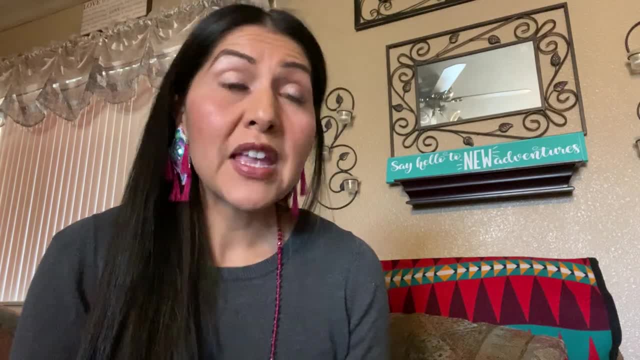 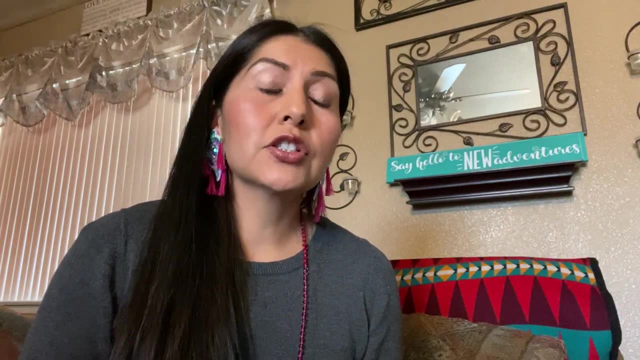 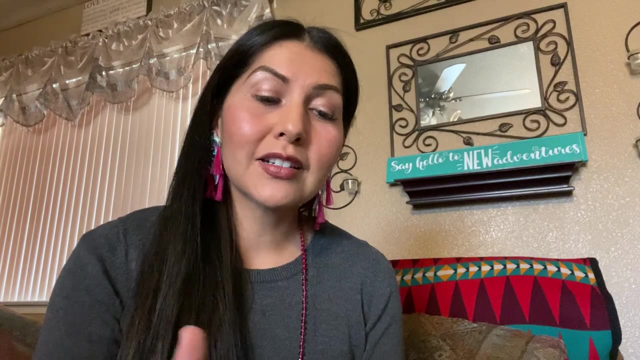 he chose to label them are not exactly what we would say them, but here's what i will tell you about one of those resources. they are a collection of songs that probably are very much so from the tribes. however, you steal um with the vast knowledge that i know about native american music. i know who.